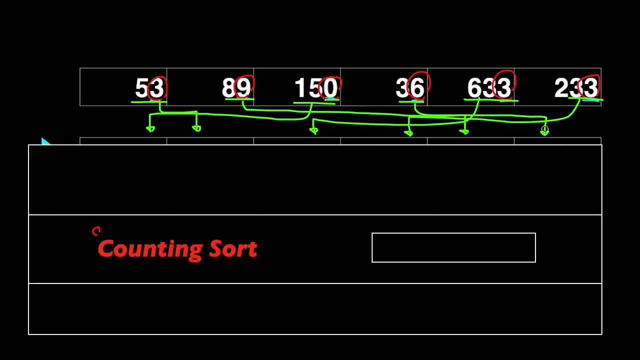 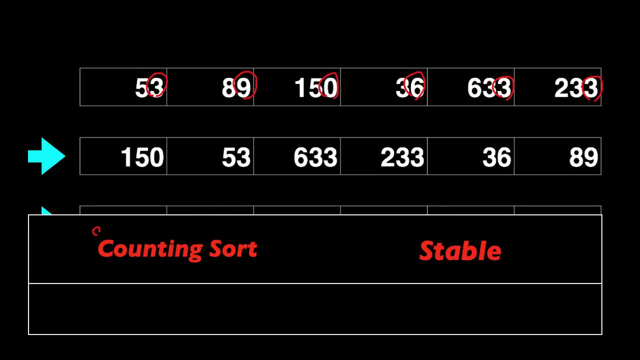 that until the very end, And the key thing to remember here is that counting sort is a stable sorting algorithm, And so the values with the same keys- in this example 53, 633, and 233,- they appear in exactly the same order in the sorted array as they do in the original array. 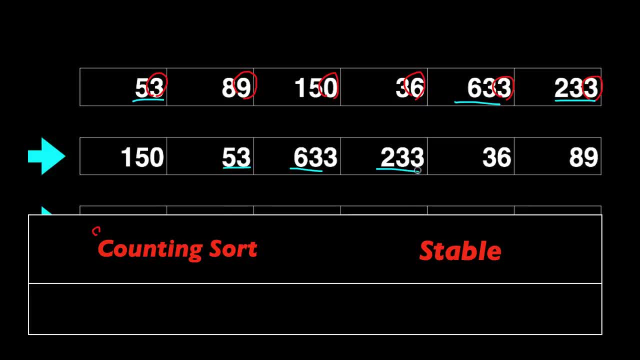 And so we're going to keep going like that until the very end. And the key thing to remember here: And it's really important to use a stable sorting algorithm as a subroutine for radix sort, because if we used an algorithm that's not stable, it just wouldn't work. Now the second step in. 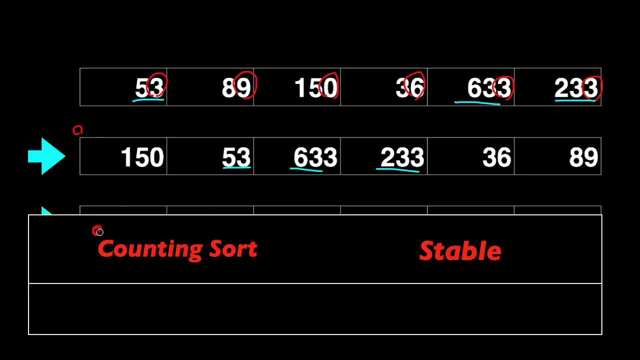 radix sort is sorting this new array using counting sort, again with the second last digit in each number as the key this time. Once we do that, the new sorted array will look like this, And we're going to repeat the same procedure with this new array, And this time we're going to use 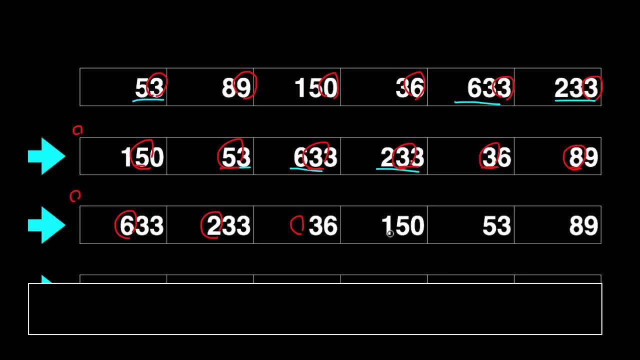 the first digit as the key And we're going to use the second last digit as the key, And we're going to use the third digit as the key, And you'll notice that there are some numbers without any number in that place, So we'll just use zero as the key for those numbers. Once that's done, the whole array is. 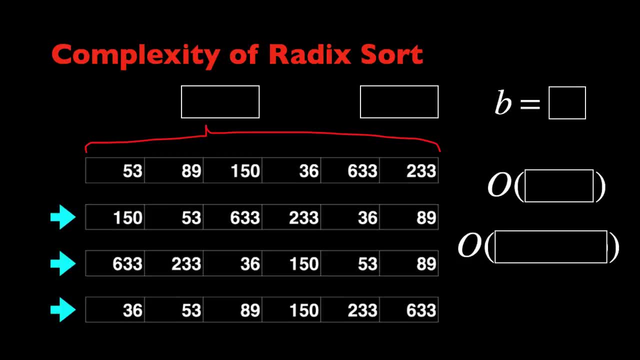